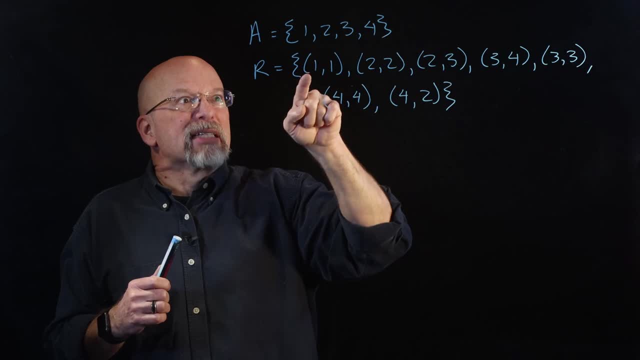 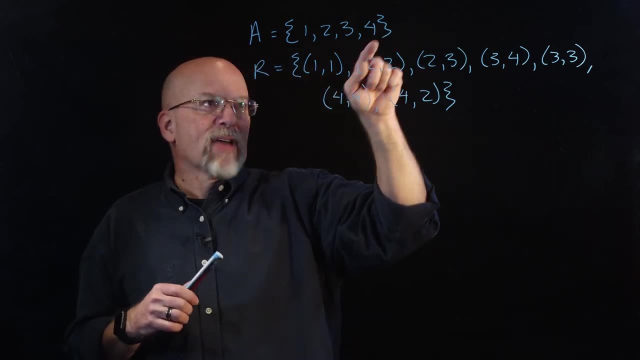 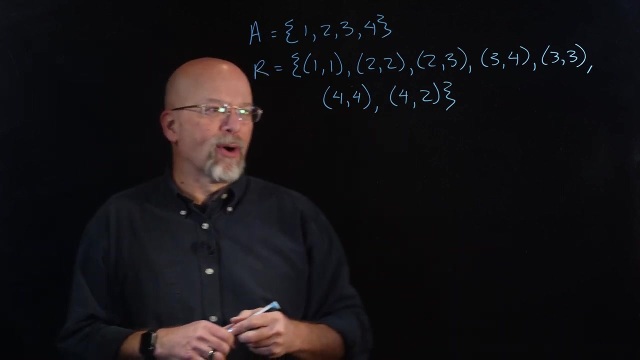 says that for every element of A that the that element is is related to itself in the subset R. For example, if A had the element five, this subset R would not be reflexive because it would be missing five comma five right Now. it helps sometimes to be able to. 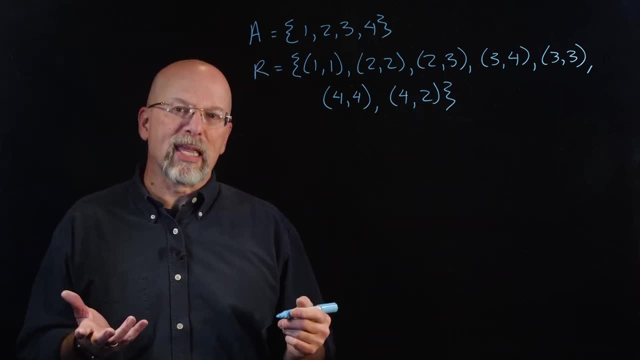 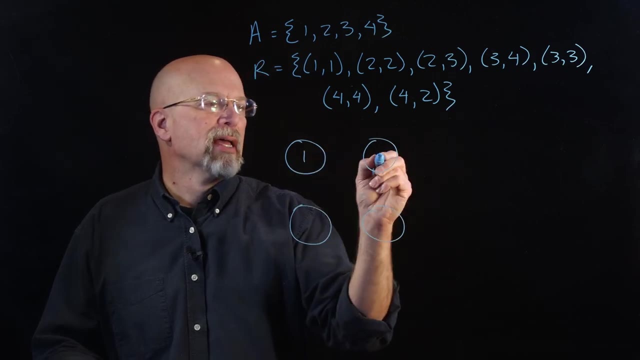 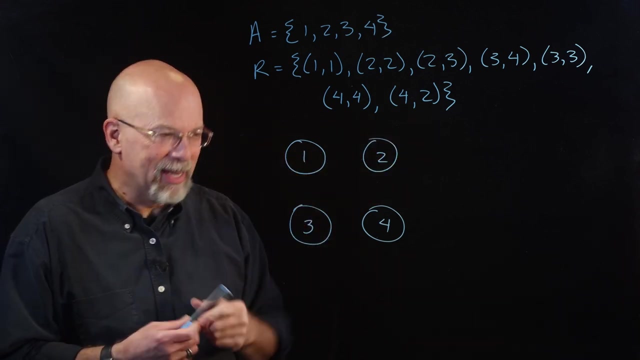 look at these things, And we talked about two alternative ways of looking at relations in the last lesson, Remember. the first one was the directed graph, And so we had. every single element was identified with its own vertex: the circle with the element name inside of it. 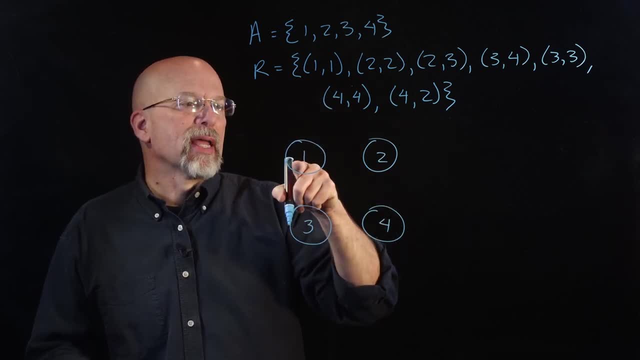 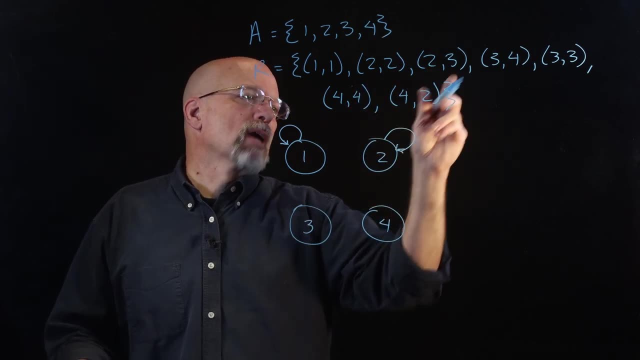 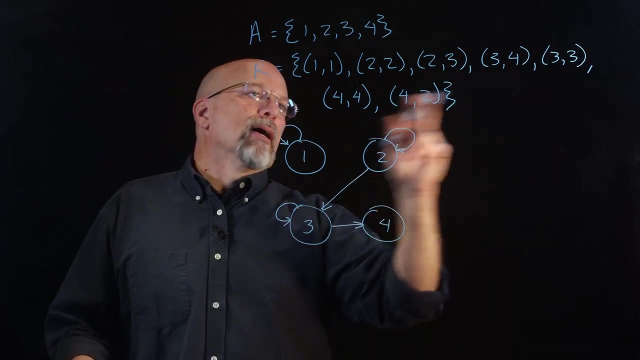 Well, the arrow indicated the relation right. So we had one comma one. that's just an arrow back to itself, right. Two comma two. arrow back to itself: Two comma three. let's see, there's an arrow: three comma four. There's an arrow: three comma three, four comma four and then four comma. 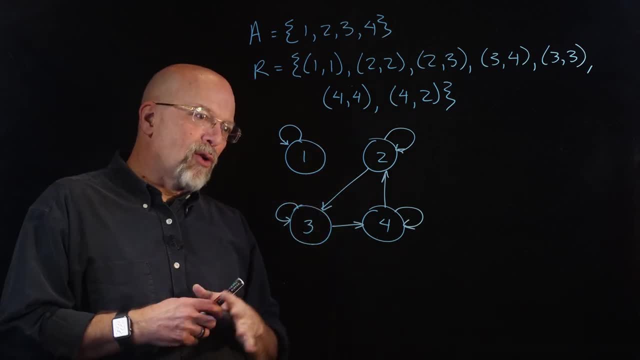 two. All right, So there is our representation And notice, nothing ended up going to one. sorry about that, But the key is is we want to have I'll call it a trajectory here, but we'll call it a polynomial, And we want to have a value that denotes: is it a value? Is it a value? Is it a value? 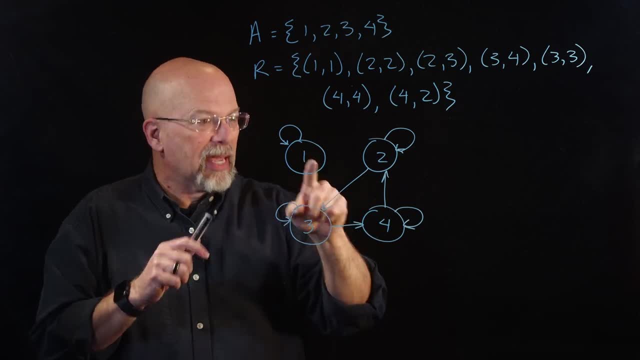 Well, the key is that: is it a value Or is it a value? Well, the key is: is it a value? That's the key thing. when you look at this representation, every single element of A, all of these vertices, have an edge. 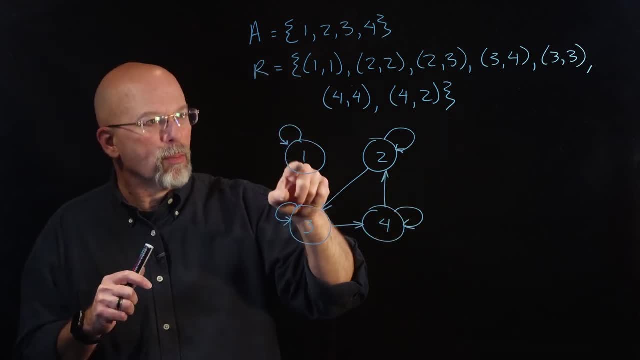 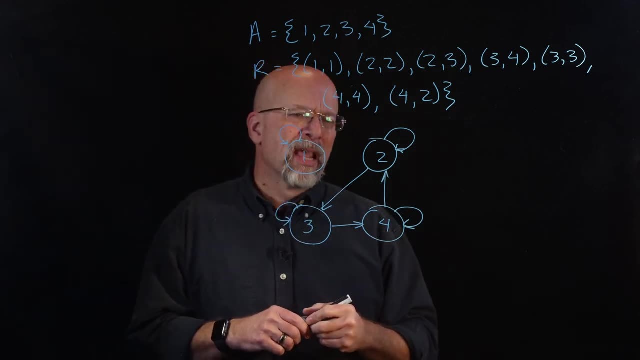 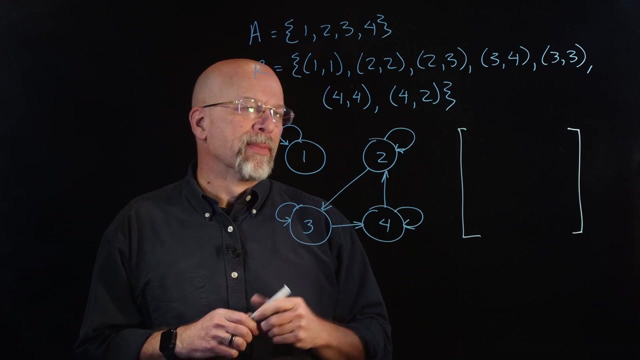 that goes back into itself. So this loop, if every single element has this loop, that indicates that it is a reflexive, it's a reflexive relation. But remember, we also talked about using a matrix in order to represent our relation And once again, this is not part of the matrix, It just shows. 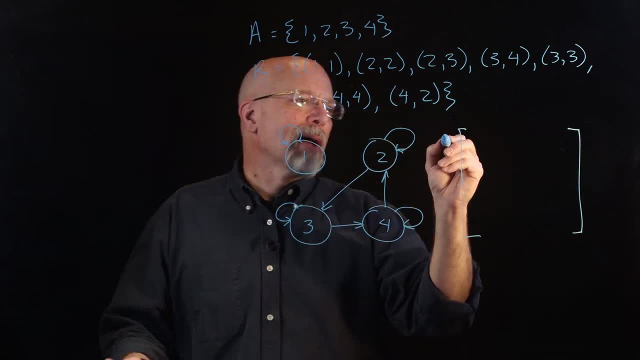 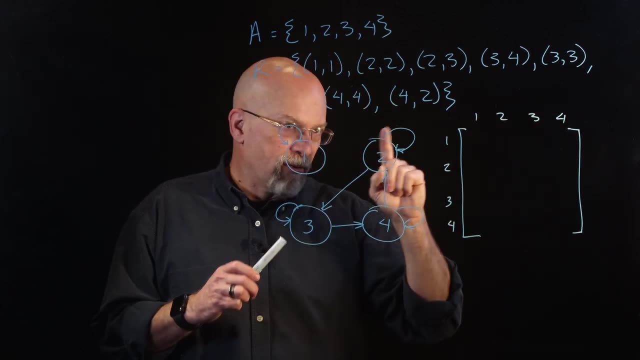 maybe helps us figure out what the matrix should look like. I'm going to number the elements: One, two, three, four. One, two, three, four, And so if one has a relation is related to one, we put a one. 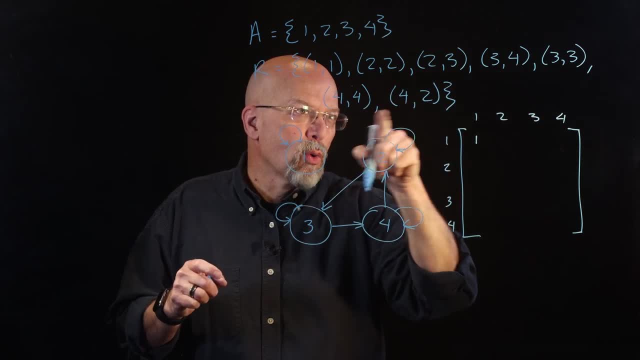 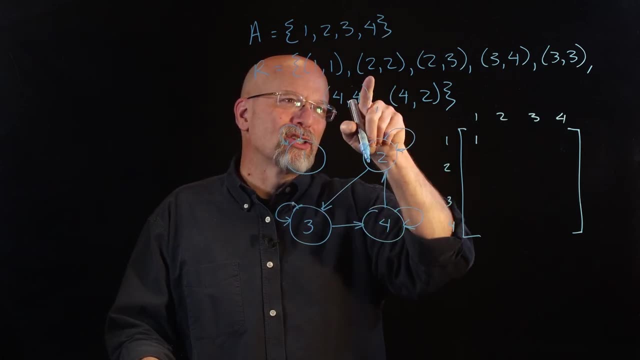 there. So every one of these pairs, every one of these ordered pairs, has a one in the matrix reflecting what that- no pun intended- what that relation is. So two comma two, that's a one there. Two comma three, so two. 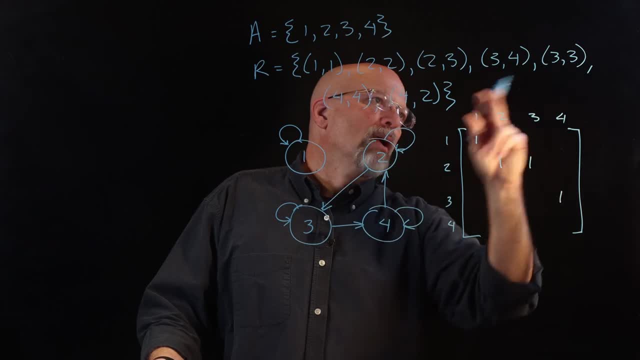 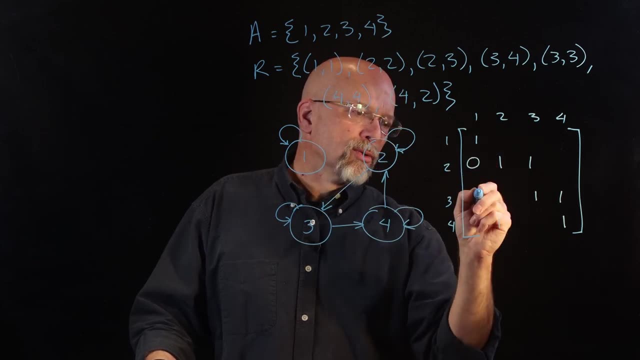 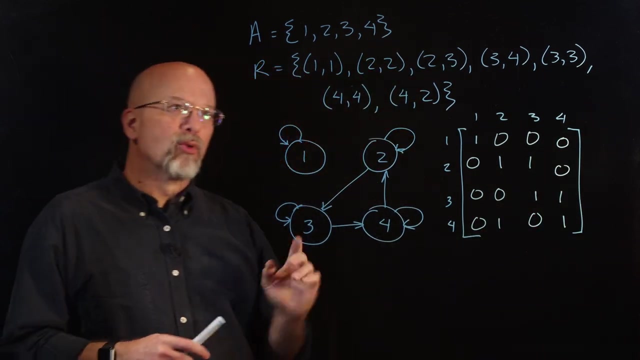 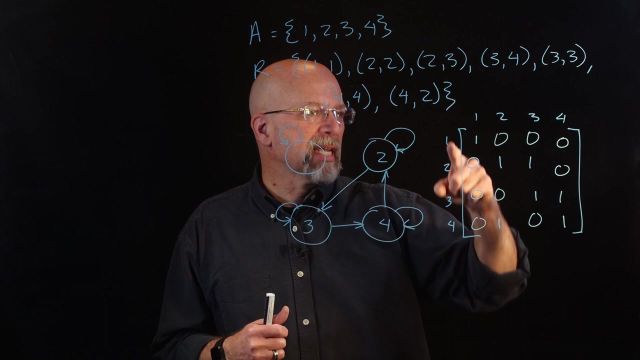 Two comma three, three comma four. right Three comma three, four comma four, and then four comma two. Zeros everywhere else. And so here is our matrix representing the relation R. And how do we figure out reflexivity from this matrix? Well, it's pretty easy. There are ones on the diagonal. 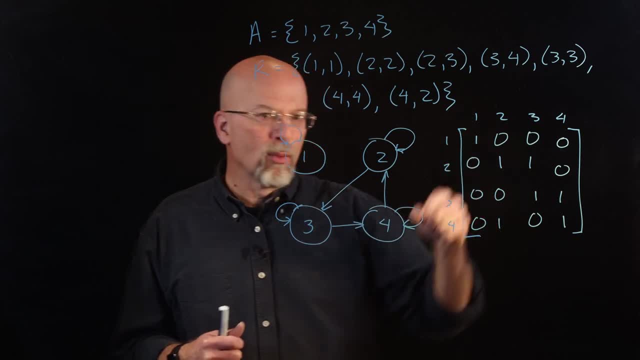 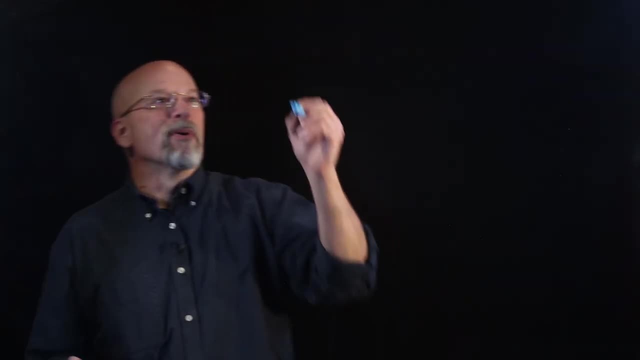 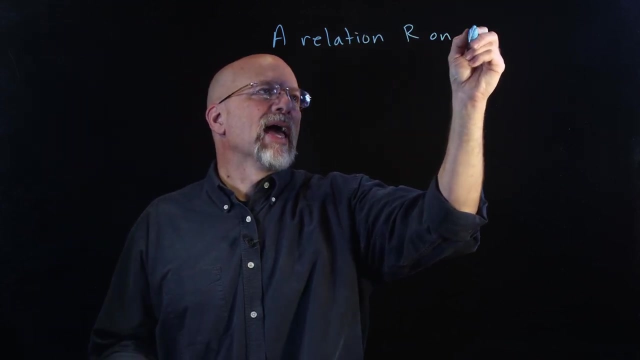 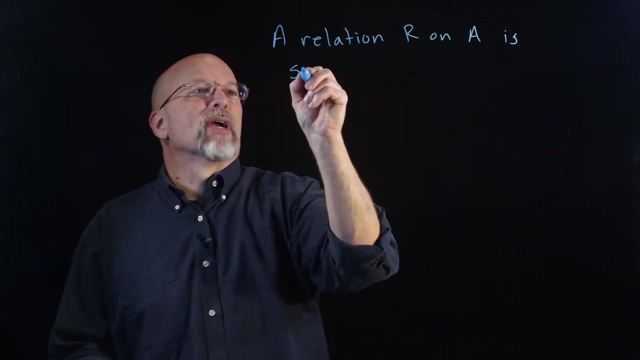 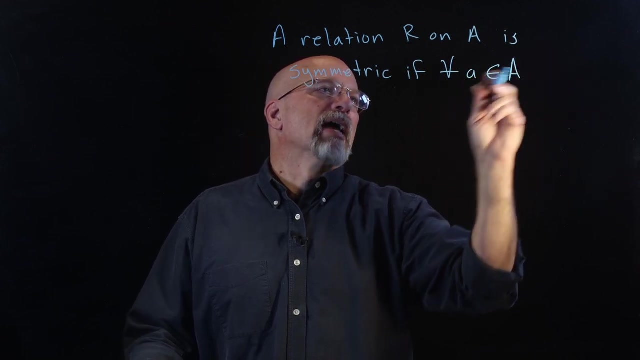 If there is a single zero on this diagonal anywhere, we don't have the reflexive property, We have another property, the symmetric property. So a relation R on A- once again that's a relation which is a subset of the Cartesian product of A cross. A is symmetric if for all A in A, for all little a in capital. 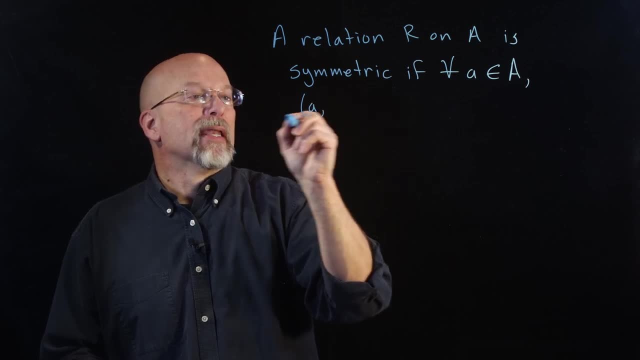 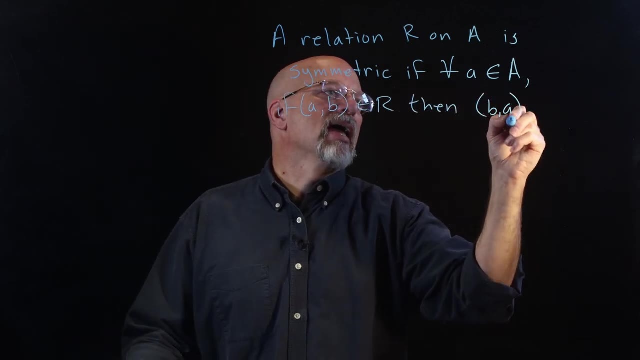 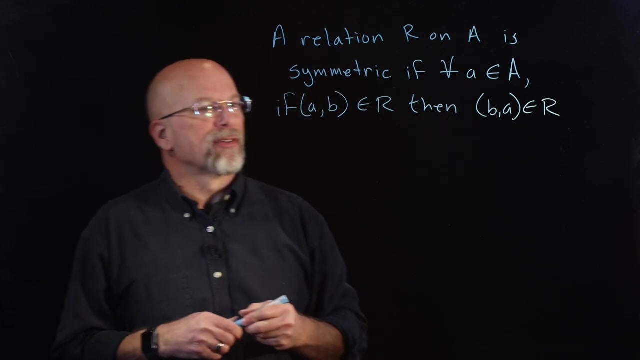 A, then if A comma B is in R, then B comma A is in R. All right, Now how do we do that graphically? How do we show that graphically? Well, what we've got, let's go ahead and do the directed graph first. 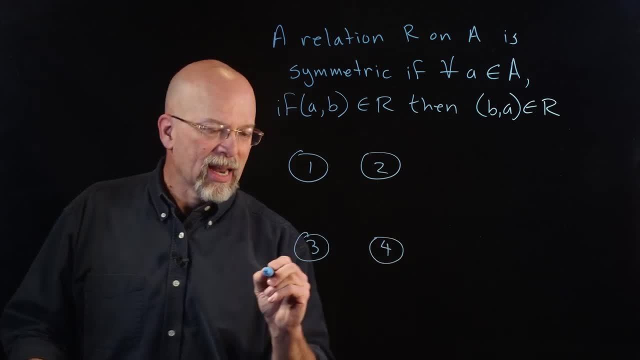 So we have one, two, three, four, And let me know, let me go ahead and define another relation here. the one before was notкогоinnual, was notreflexive, was not сказать, but the one before was not нflexive. 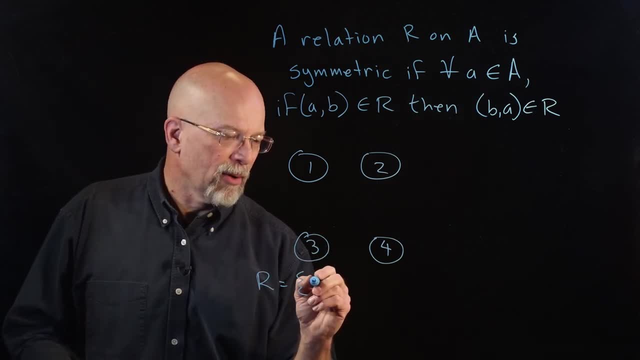 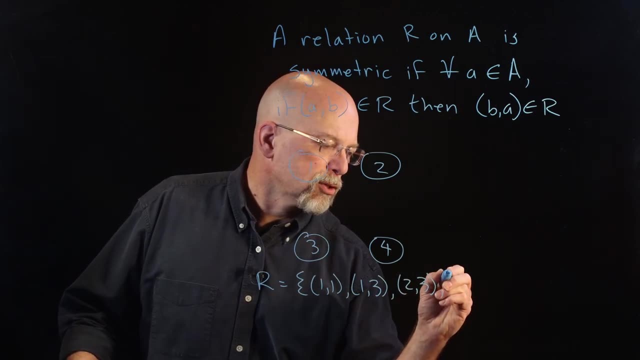 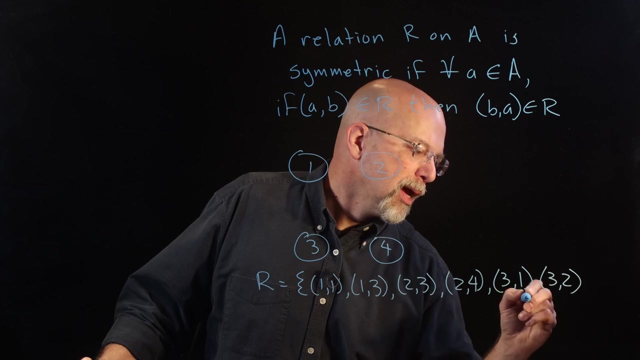 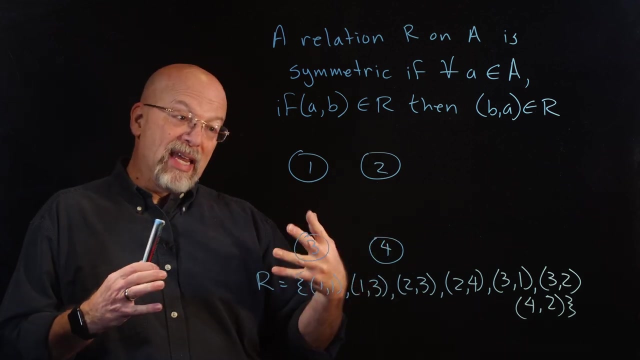 relation here. The one before was not reflexive. And how about we do 1, 1,, 1, 3, 2, 3, 2,, 4, 3, 1,, 3,, 2, and we'll also add 4, 2 on here. All right, And so once again, we create an edge from each one. 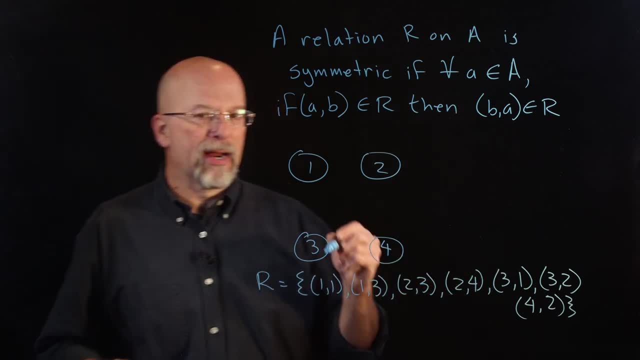 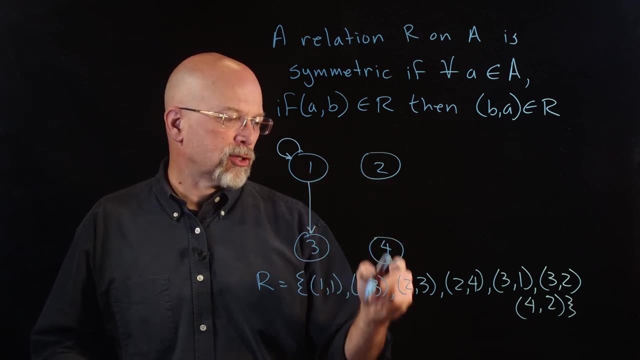 of these vertices to a vertice representing each one of the ordered pairs. So we'll start out with 1, 1, and then the ordered pair 1 to 3.. So we got 1 to 3, and then 2 to 3.. All right, And then 2 to 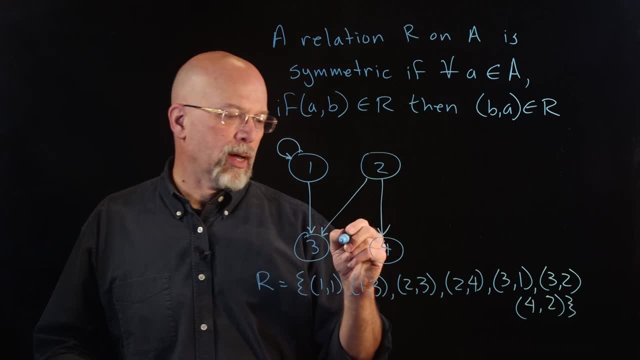 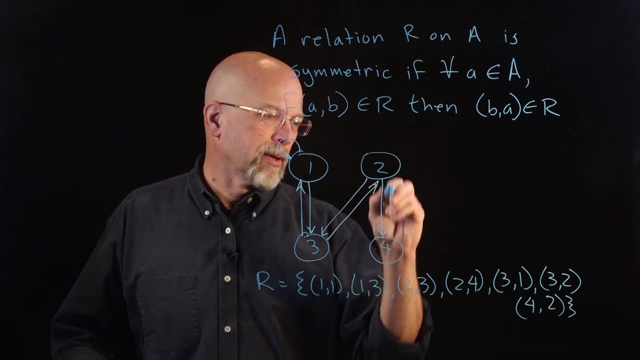 4. So 2 to 4,, 3 to 1.. So 3 to 1,, 3 to 2,, 3 to 2, and 4 to 2.. All right, Now does this have the? 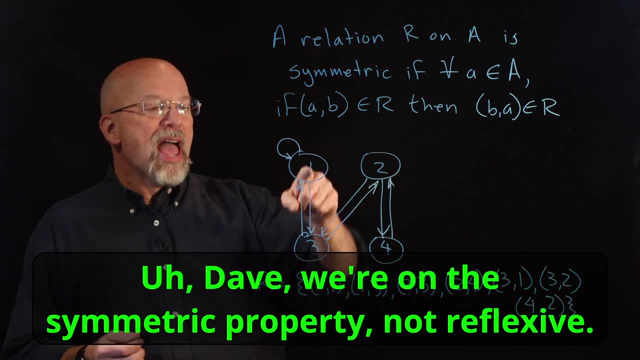 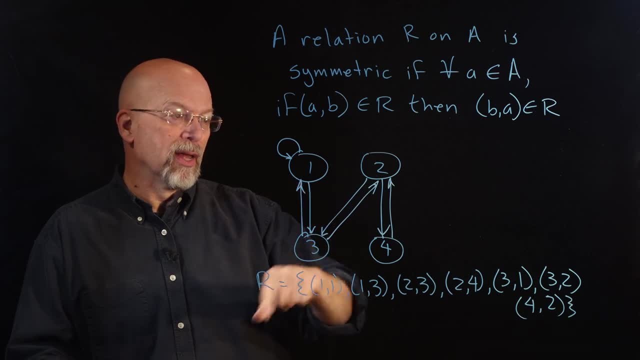 reflexive property. Right With the direct graph it's pretty easy to tell. Every arrow going one direction must have an arrow going in the opposite direction, And so we've got an arrow from 1 to 3 and an arrow from 3 to 1.. We've got 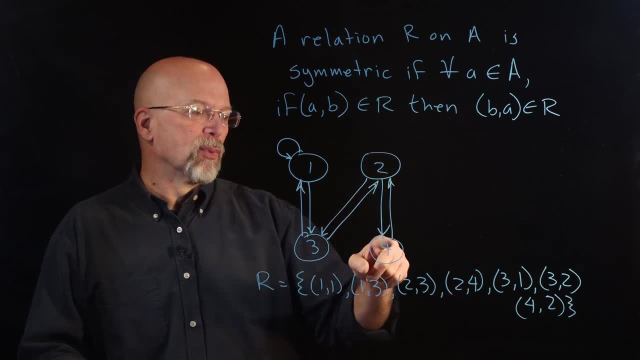 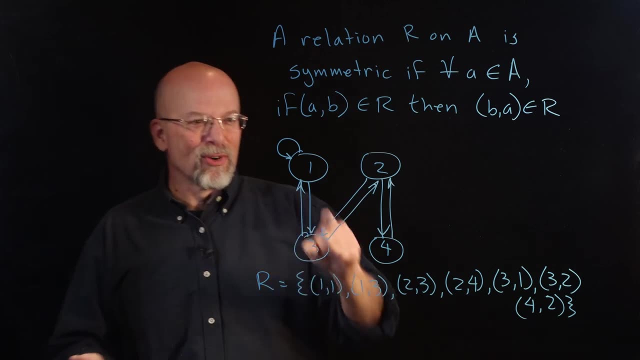 edge from 2 to 3.. We've got an edge from 3 to 2.. We've got an edge from 2 to 4.. We've got an edge from 4 to 2.. The only one that doesn't have a buddy that's going in the opposite direction is 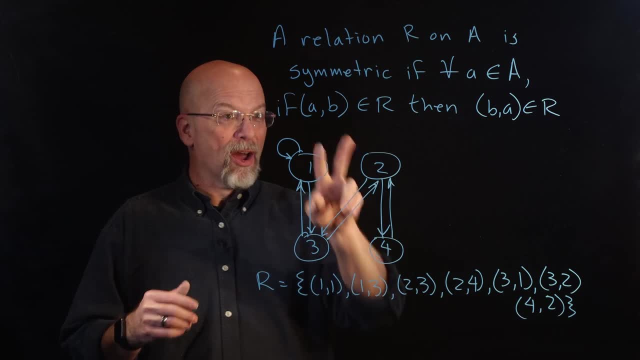 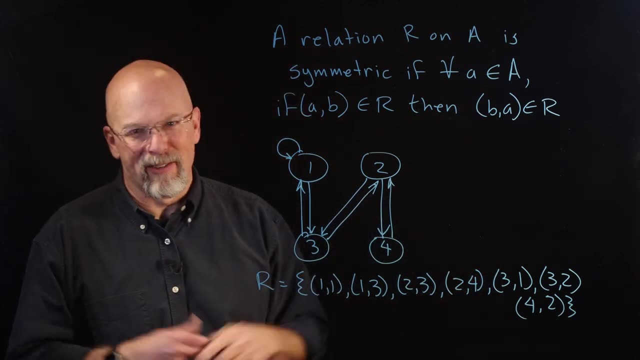 this one, that's going from 1 back to 1.. Once again, though, if we have, if 1, 1 is in R, then 1, 1, 1 is in R. Yes, we have both directions, So this relation, it turns out, is symmetric, And we can. 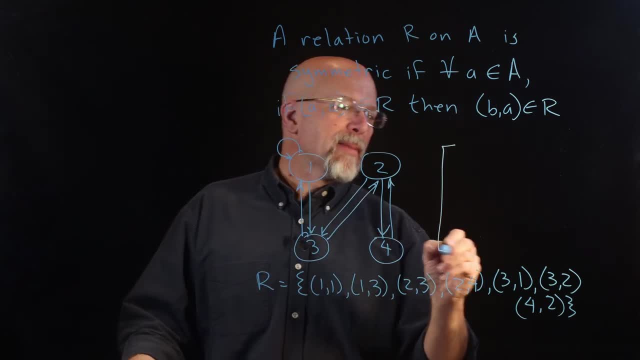 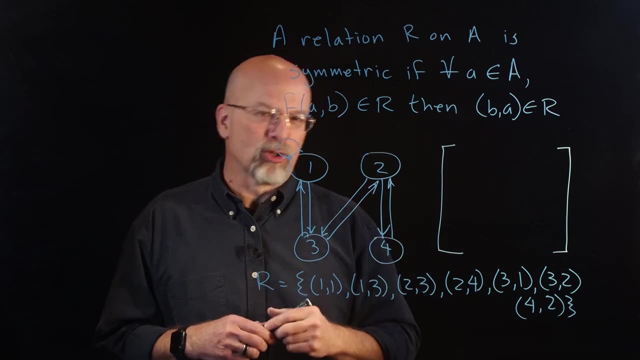 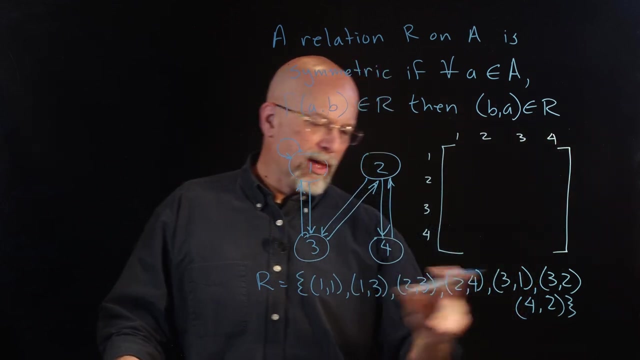 see that from the die graph, But what about from the matrix? Can we have? is there some way to look at the matrix and be able to tell right away that we have a symmetric relation? Well, let's go ahead once again and we'll represent our set with the matrix. So I've got 1, 1,, 1, 3.. 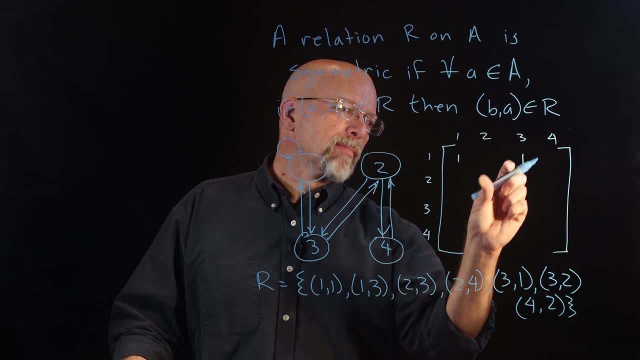 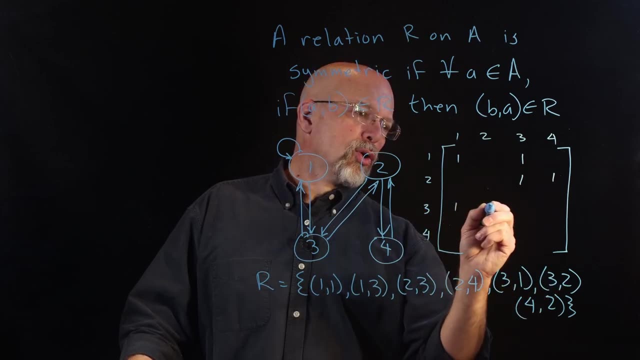 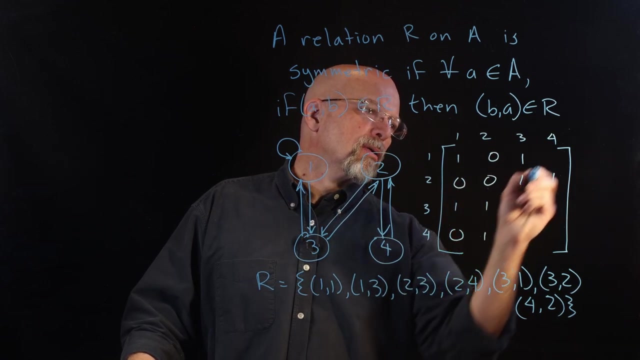 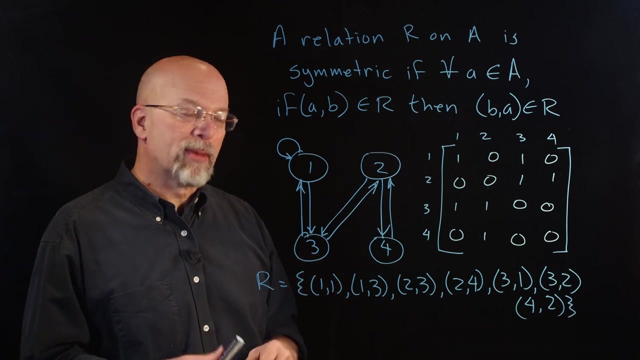 2, 3.. Whoops, 2, 4.. 3, 1.. 3, 2.. And then 4, 2.. All right, Zeros everywhere else. All right. Now how is the matrix going to help us identify whether a relation is symmetric or not? 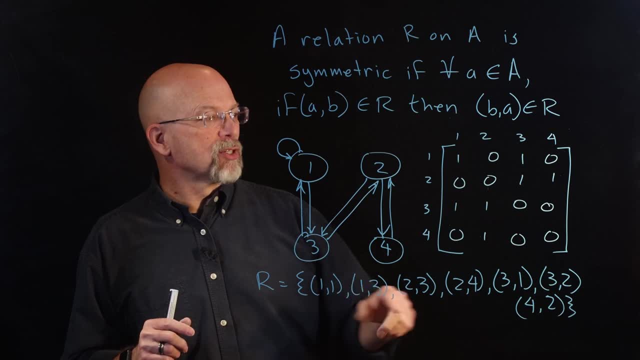 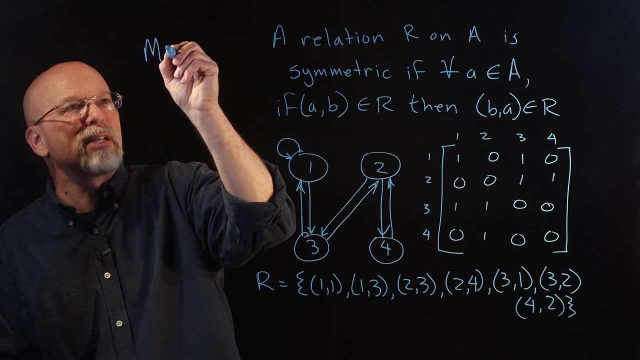 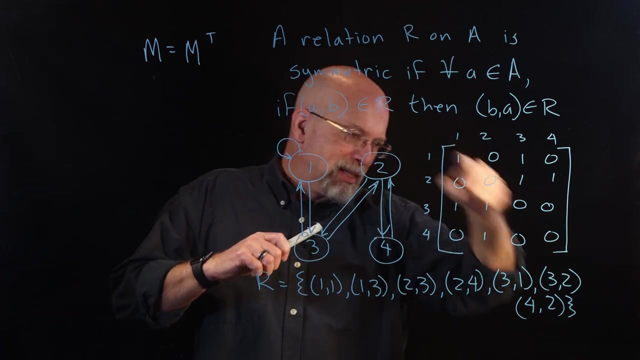 Well, it's pretty simple actually. If you remember our study on matrices, we had this property of a matrix being symmetric and that definition for a matrix being symmetric. a matrix m is symmetric if it is equal to its transpose, and the transpose was: we flip it over the diagonal. so 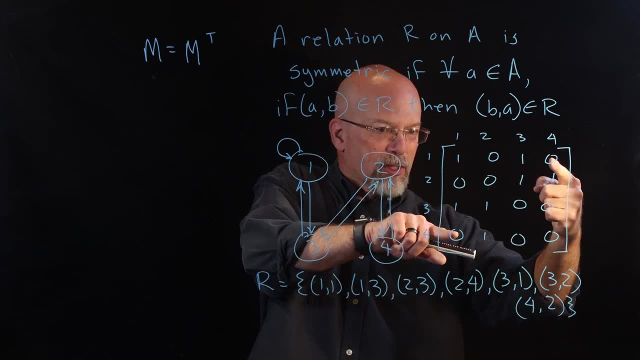 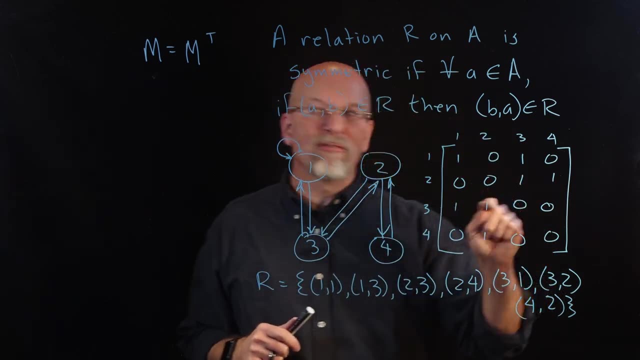 if we flip this over the diagonal, you'll notice that everywhere there's a zero, there's a zero in the transpose, and everywhere there's a one, there's a one in the transpose. so this matrix is, in fact, uh, symmetric, because we can flip it across the diagonal, and it's equal to the original matrix. 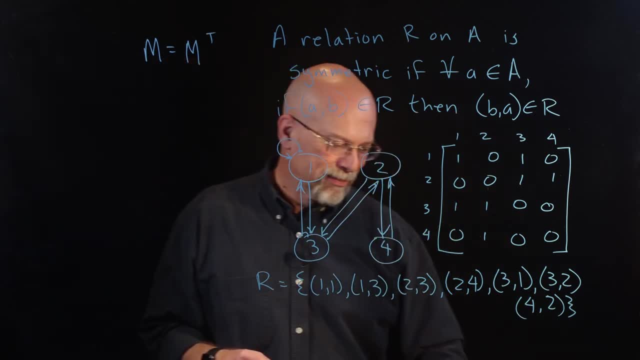 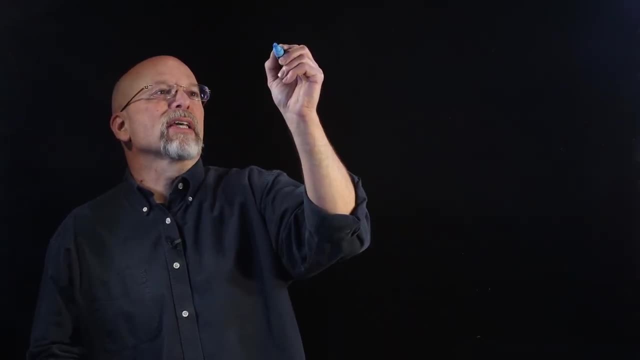 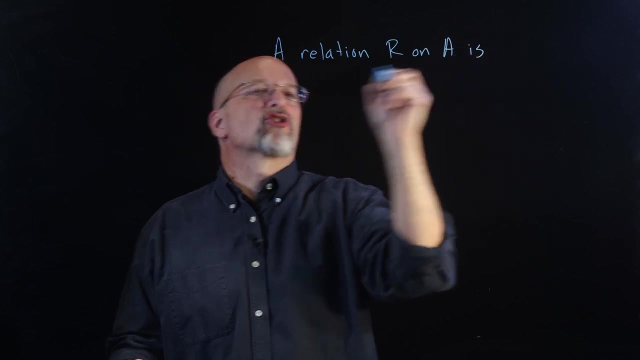 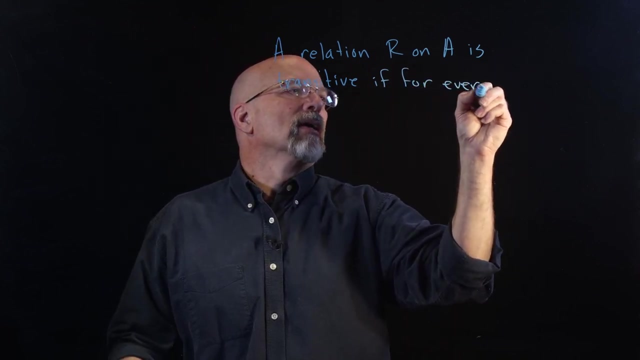 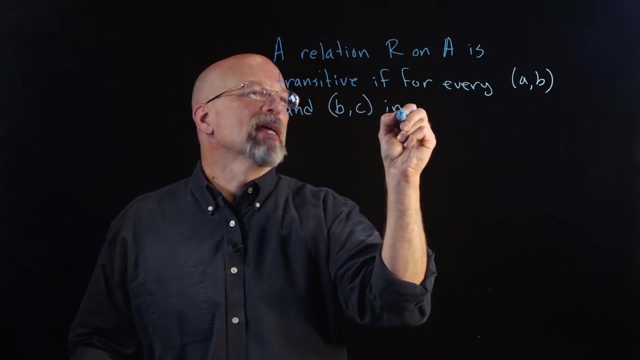 that means that our relation is also symmetric. the next property we're going to look at is the transitive property and basically we have a relation: r on a is transitive if for every a comma b and b comma c in r, uh, a comma c is in r. 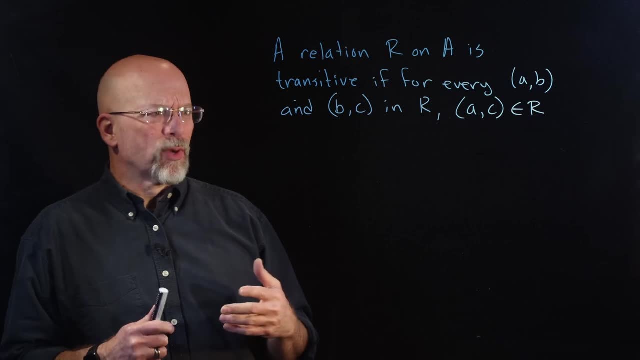 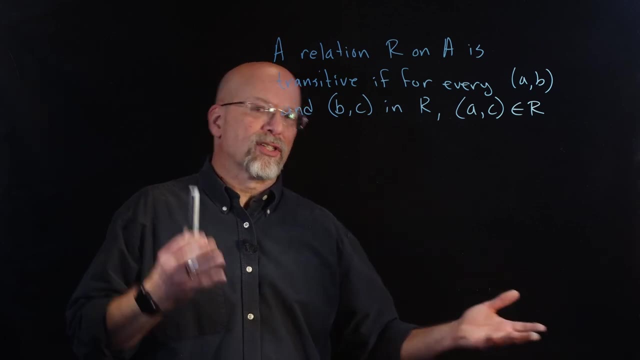 huh yeah, transitive property. i mean you're used to using this with like equality, right, if a equals b and b equals c, then a equals c. if a is greater than b and b is greater than c, then a is greater than c, but it's not true for everything. for example, if a is equal to negative, b and b is. 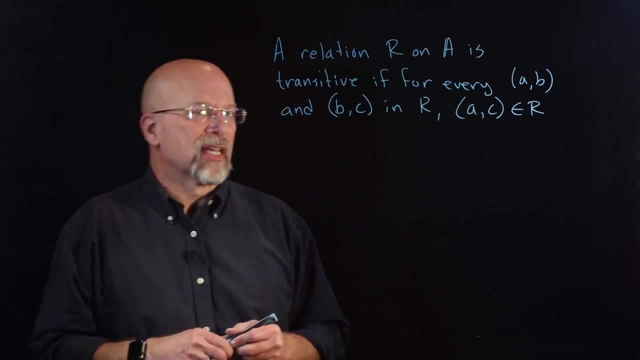 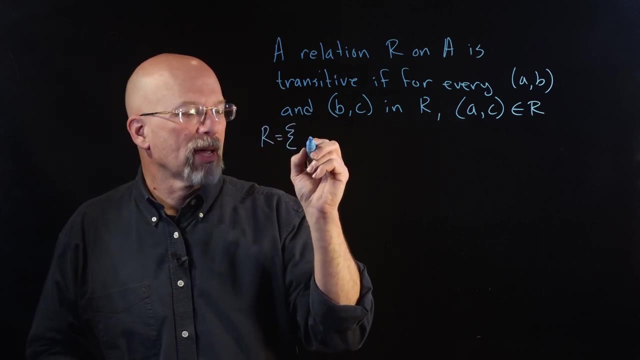 equal to negative c, then a is not equal to negative c, then a is equal to negative c if a is not equal to seen. So let's take a look and see if we can't figure out what a transitive relation looks like, And let's start off again with another example. How about R is 1, 1.. It contains 2, 2.. It contains. 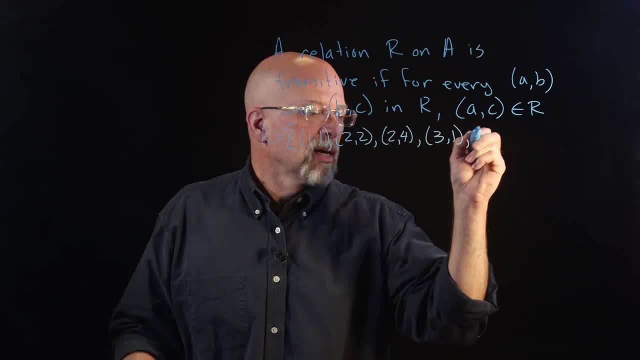 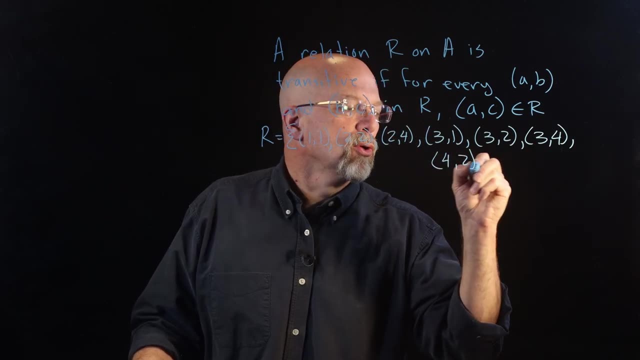 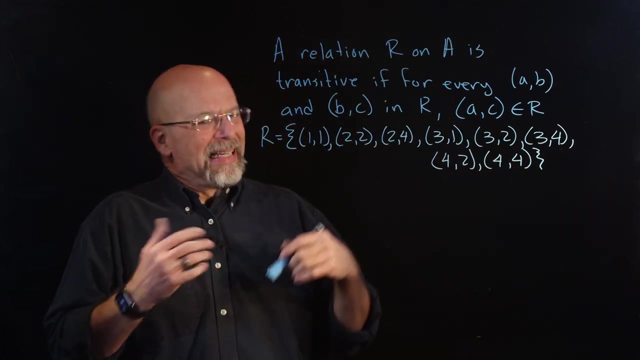 2, 4.. 3, 1., 3, 2.. 3, 4.. 4, 2. And 4, 4.. Now, what we're going to find is that, whenever it comes to the digraph, it may not be obvious right away- We'll show you how to trace paths and so forth. 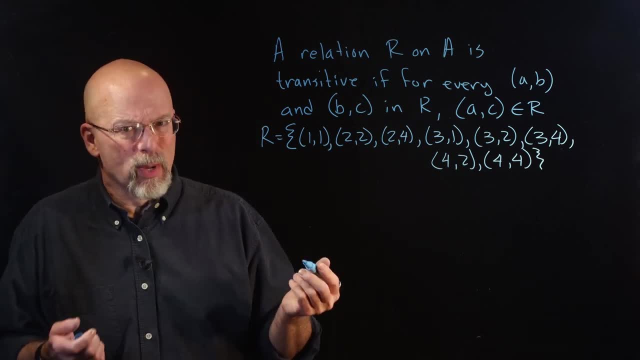 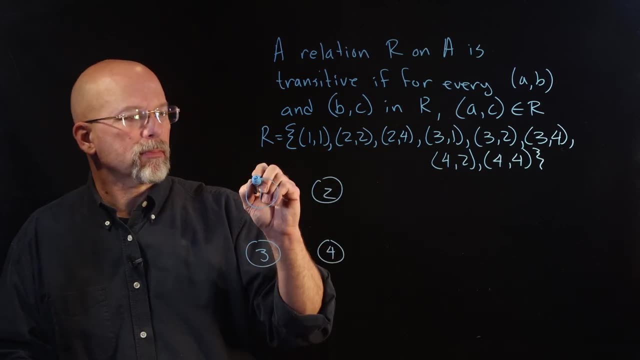 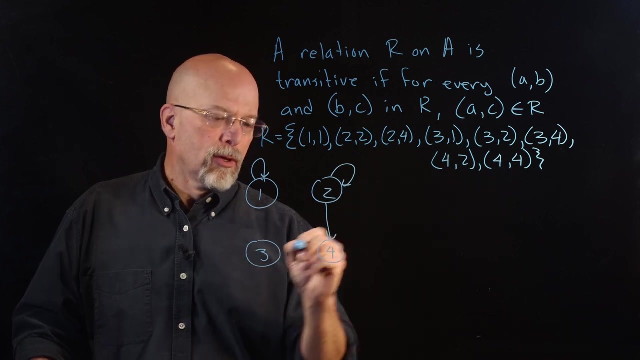 but it's not going to be as obvious, hopefully, as we would have hoped. So we've got the four elements right: 1,, 2,, 3, and 4.. And so 1 goes to 1.. 2 goes to 2., 2 goes to 4.. 3 goes to 1.. 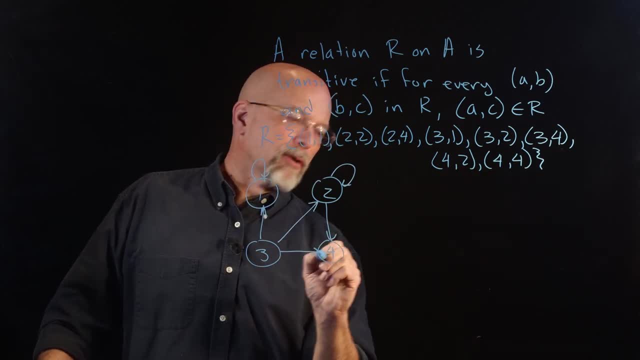 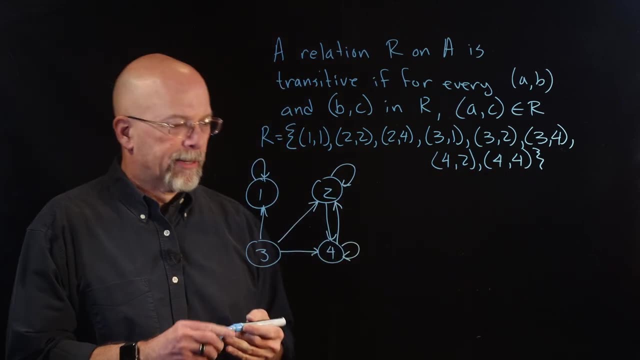 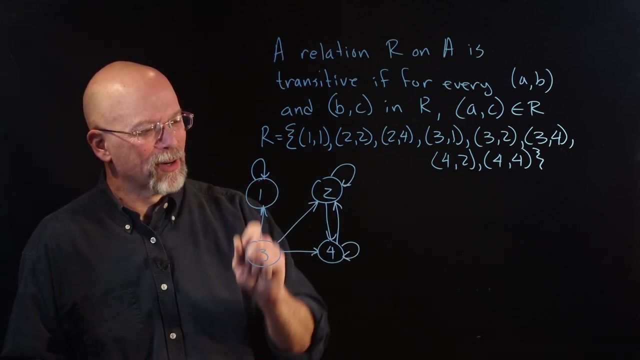 3 goes to 2.. 3 goes to 4.. And let's see: 4 goes to 2. And 4 goes to 4.. Is that right Now? can we look at this and figure out whether it's transitive or not? Well, it's going to be a little complicated. For example, 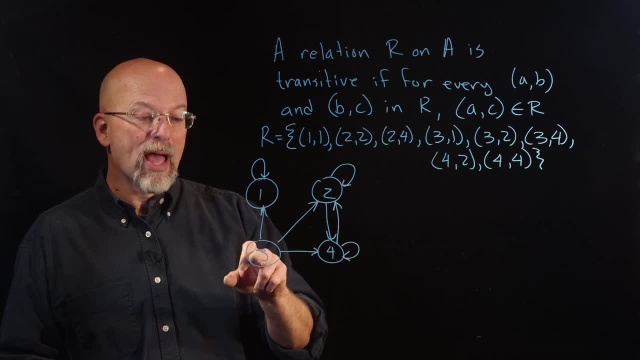 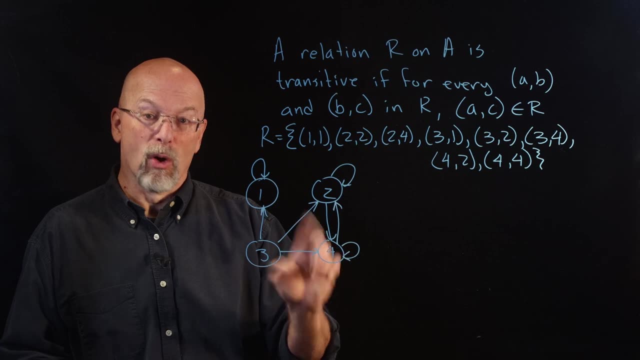 I've got a relation 3 to 1, and I've got a relation 1 to 1.. Do I have a relation 3 to 1?? Yeah, I do. I have a relation 3 to 2.. I have a relation 3 to 4.. Do I have a relation 3 to 4?? 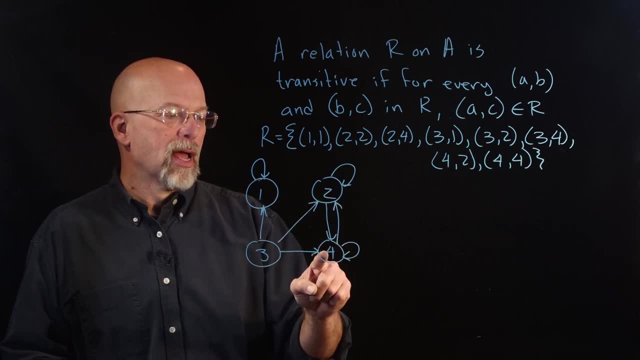 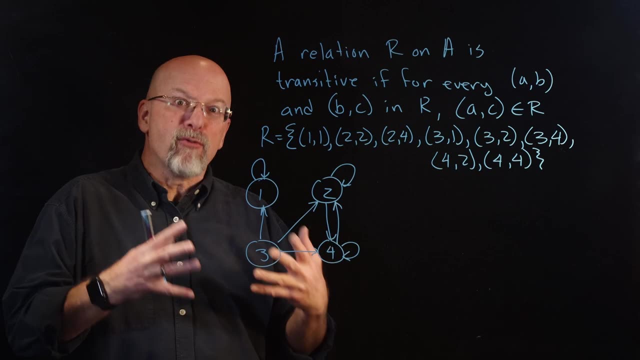 I do. How about 2 to 4 and 4 to 2?? Then 2 to 2, right, So it looks like it. but are we going to make every possible combination? Is there something we're going to miss? Well, it turns out. matrices may help us in that area. 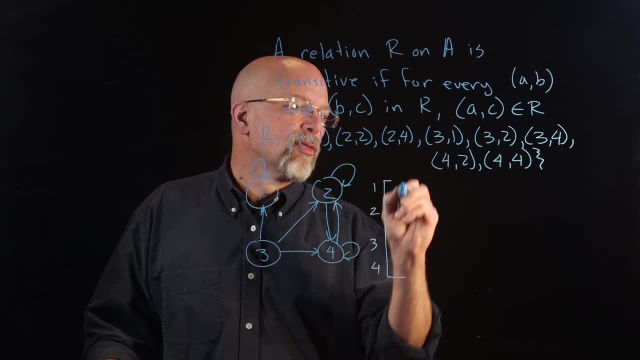 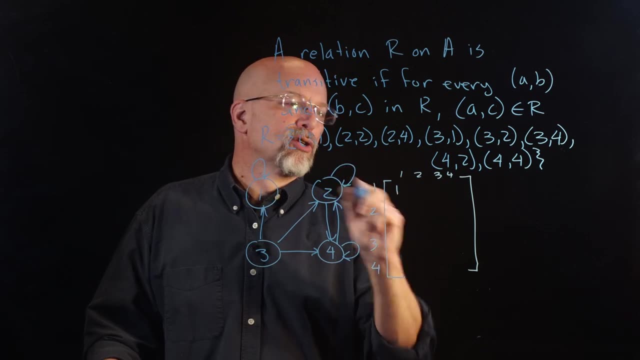 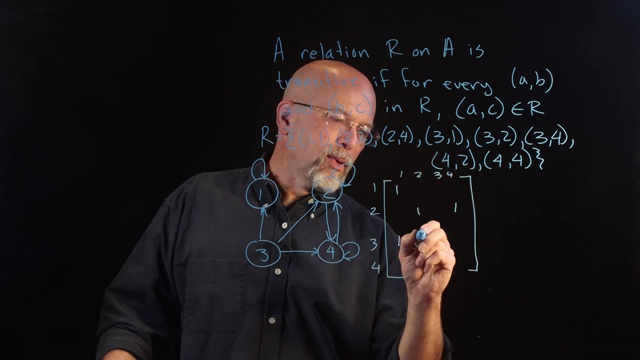 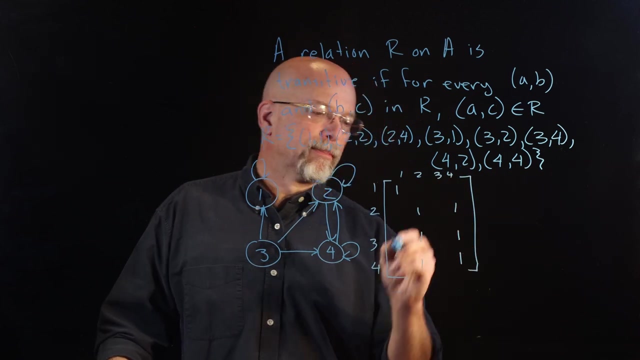 If I look at a matrix for this relation- and we'll try and get this done- 1, 1, 2, 2,, 2, 4, so 2,, 4, 3, 1.. 3, 2, 3,, 4,, 4,, 2, and 4, 4.. So there is my matrix. 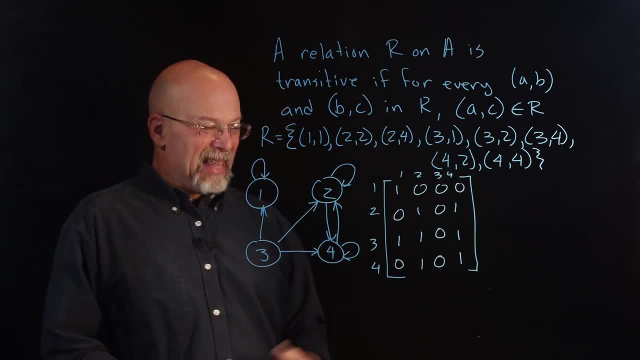 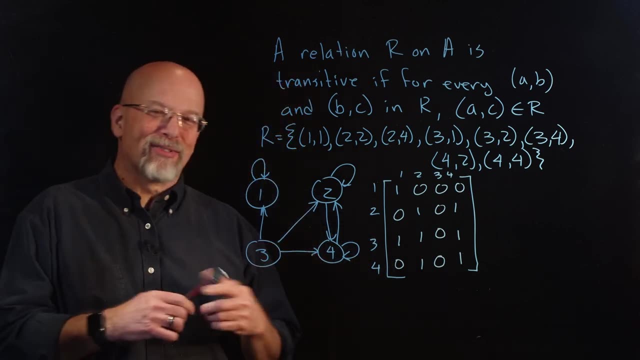 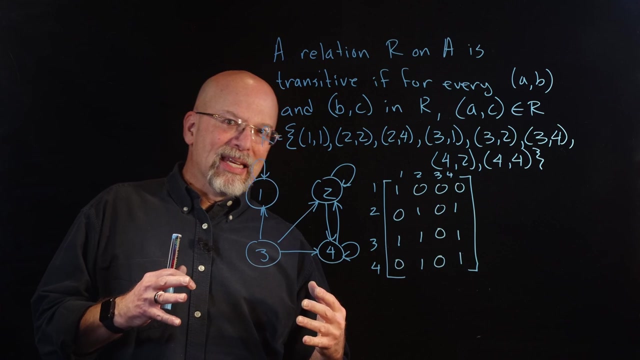 All right, Well, gosh, that matrix really is. that's no easier than the digraph. Well, it turns out that we have this property. If you look at this matrix, everywhere there is a 1, that indicates that there is a 1.. And if you look at this matrix, everywhere there is a 1,. 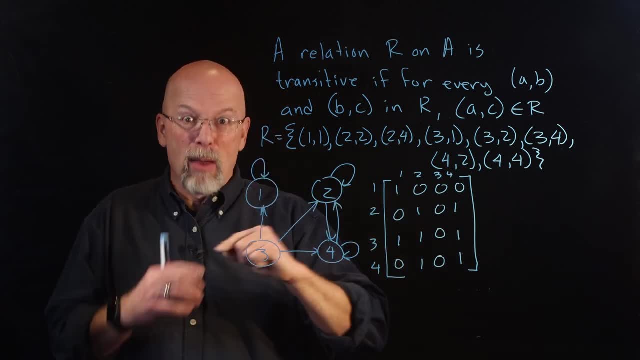 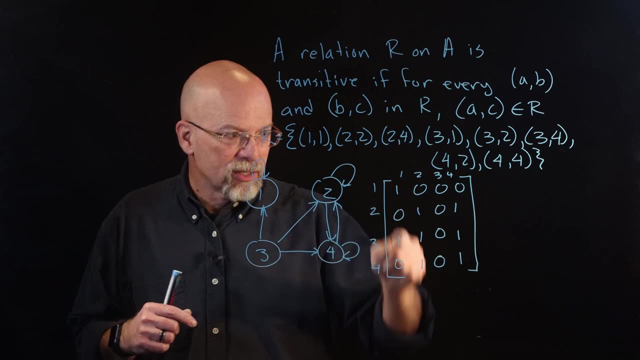 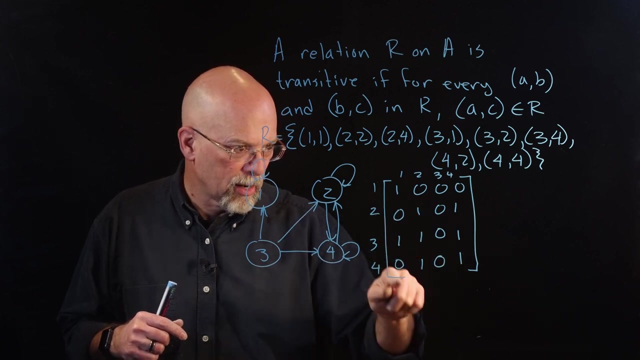 there is a connection of length 1, a path, a walk of length 1 from the row, the element that's identified by the row, to the element identified by the column. For example, this 1 right here, this 3, this 1 at 3, the row 3, column 1.. That means that we have a path of length 1 from 3 to 1.. 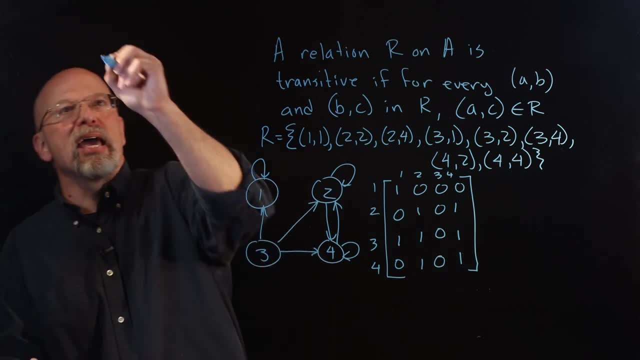 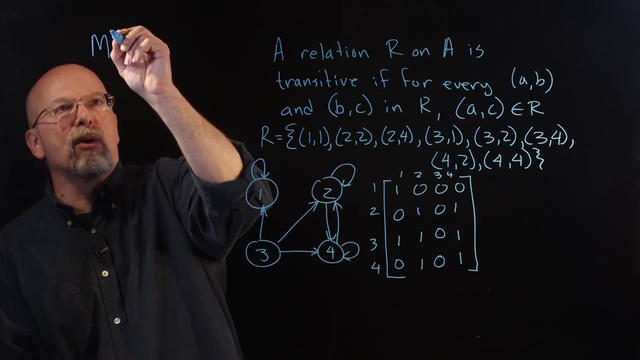 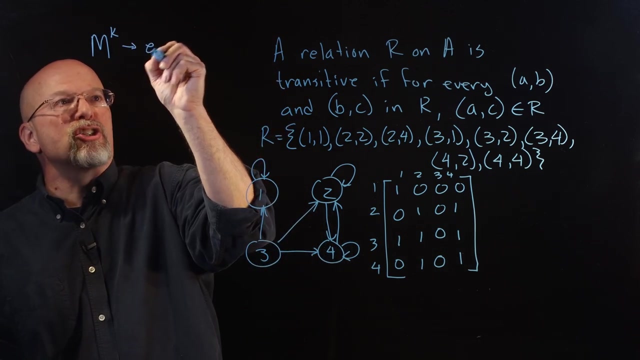 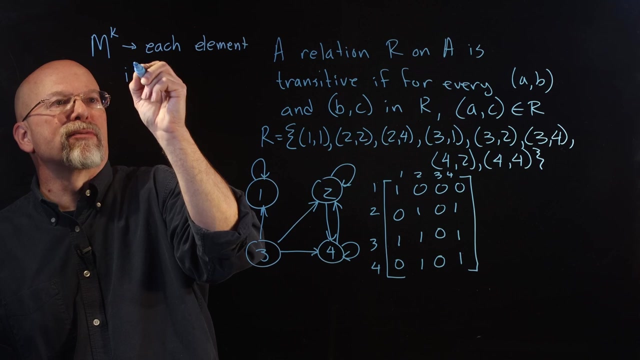 3 to 1.. All right, Well, what's interesting is that if I take the- and this is a square matrix, so I can actually raise it to different powers- If I raise a matrix to the power k, then each element identifies the number. 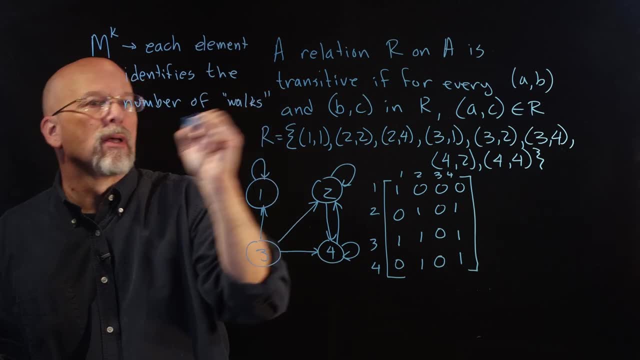 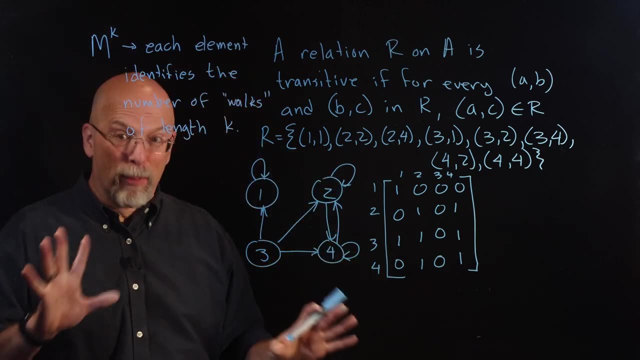 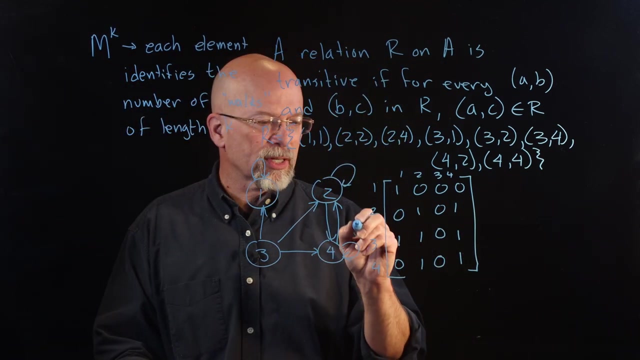 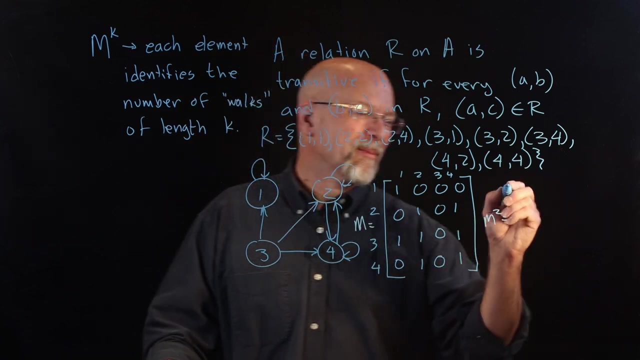 of walks or paths of length- length k- that's now the proof of this- is actually beyond what this lesson is going to cover. but let's take a look and see what happens. if this matrix right here we call this m, then m squared, and i'm just going to go ahead and write this up on the board- uh, is going to equal. let's see it's. 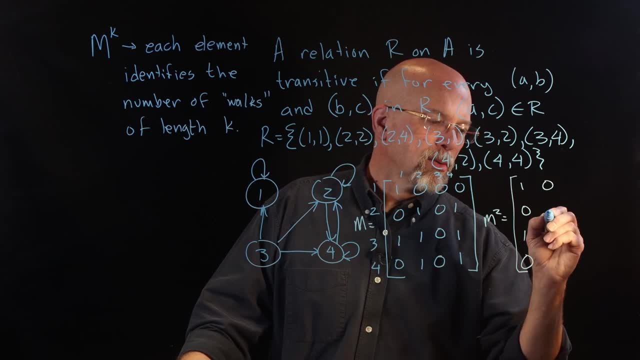 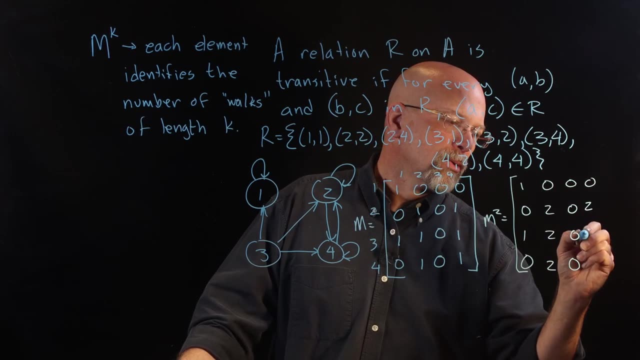 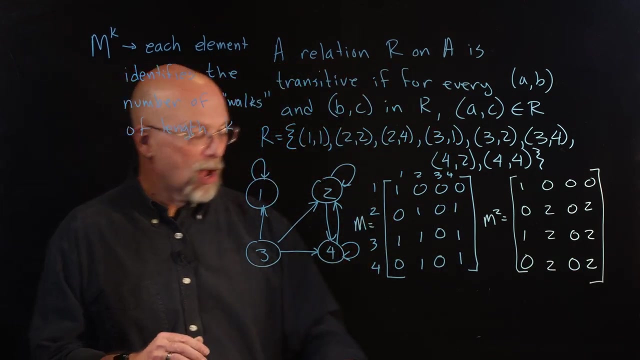 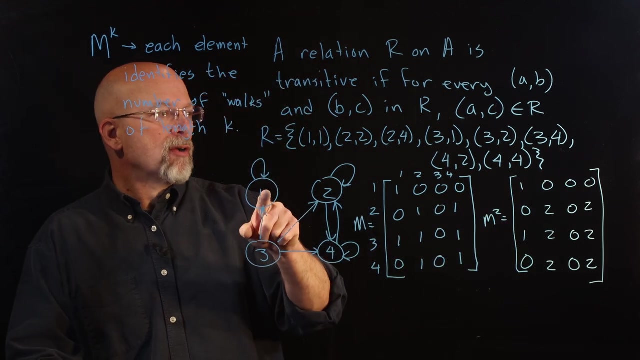 one, zero, one, zero, zero, two, two, two, then all zeros and then zero, two, two, two. i believe that that is the square of this matrix. now what this means. let's interpret this. this right here, this one right here, says that i have one length of path, two from one to one, and that path length of path. 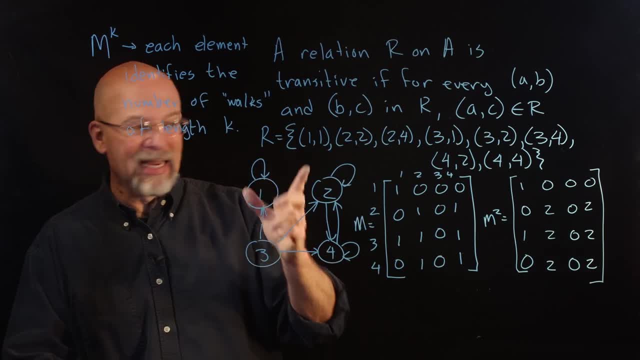 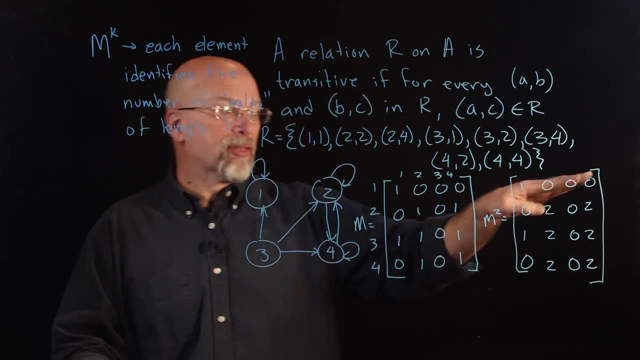 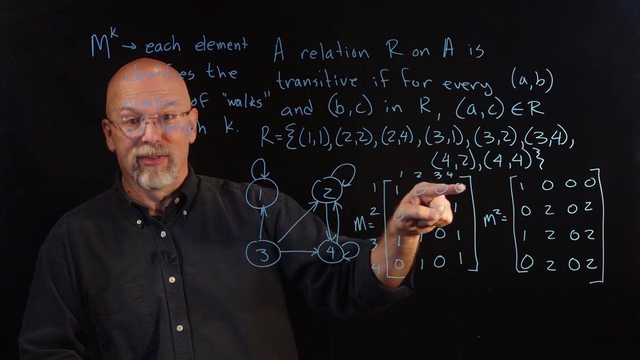 that path of length two is one two. all right, did it? uh, there are no other paths from one to one in anything of length two. so there's no way to get from one to anything over, well over- a length path of length one or a path of length two. 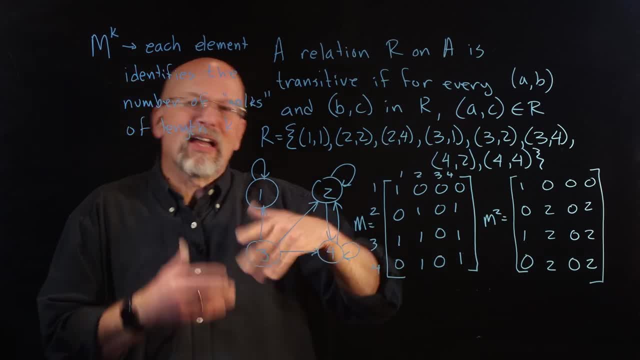 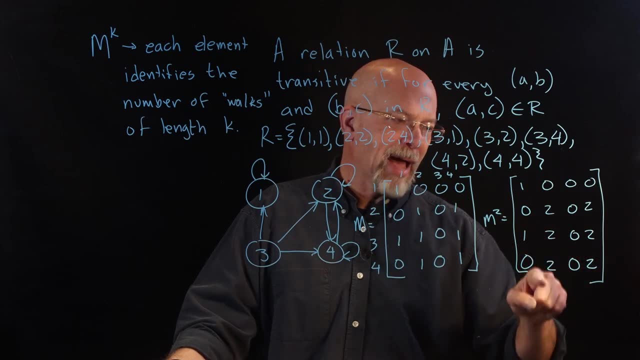 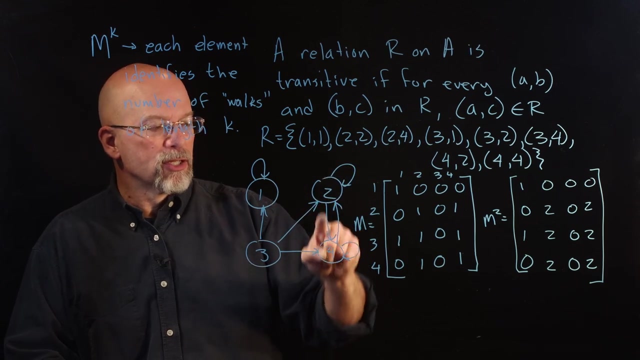 let's talk about three. can we get from three anywhere? and in fact no, let's go back to the matrix. so this right here, this element right here, says there are two ways to get from the element two back to the element two in two hops. one of them is one- two makes sense, right. the other one is to four and then back to two. that's our two. 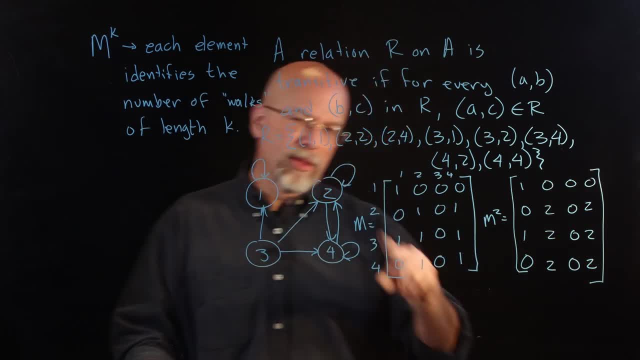 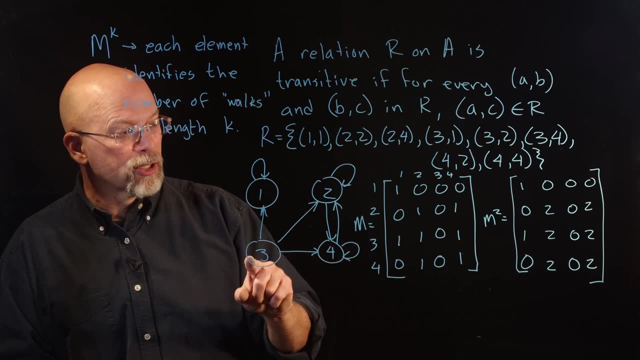 how about here? if we want to get from element three to element four? there are apparently two ways to do that. one of them is to go from three to four and then from four to four, and then. the other one is to go three to two and then two to four. now, what on earth does this have to do? 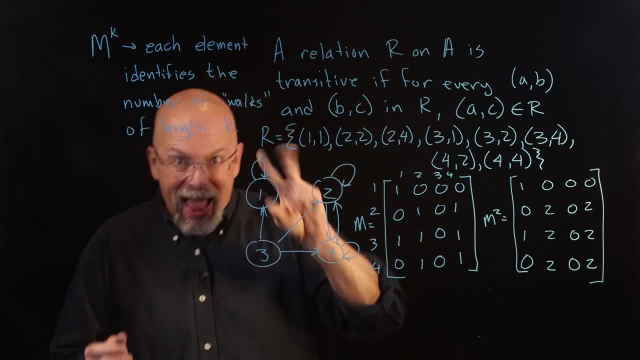 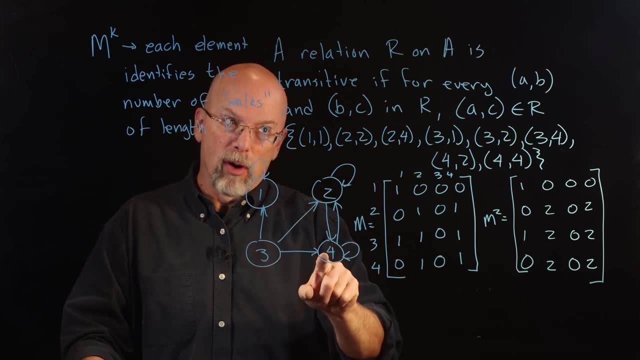 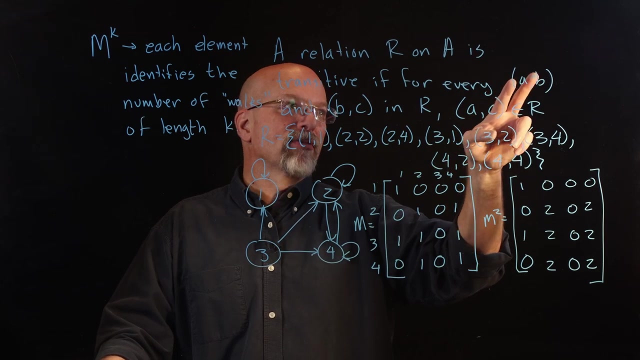 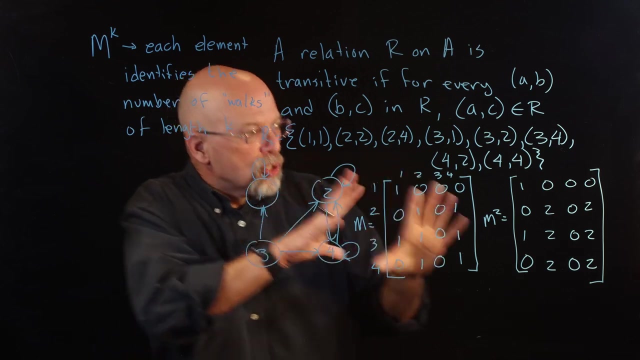 with our transitive property. well, the, the path of length two is the a comma b and b comma c. all right, so three to two, two to four. that implies that we also have a path of length one from a to c. so a path of length two a to c via b, and a path of length one a to c. so what? 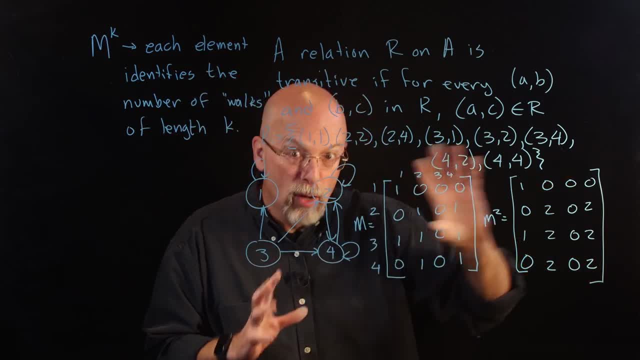 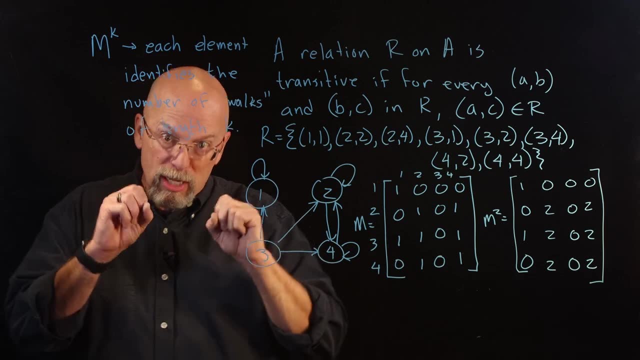 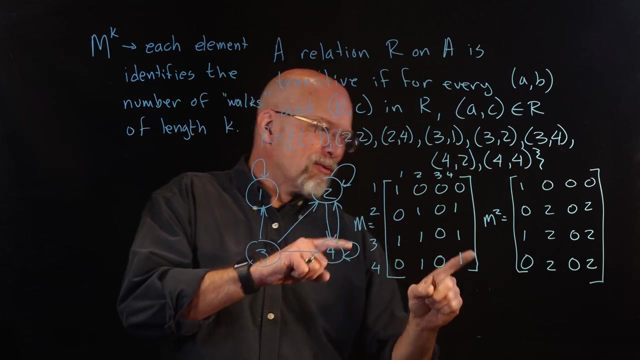 you're looking for is if there is a path of length two that is represented by this matrix squared, that represents any way to get from one node to another node in two hops, there also has to be a path of length one, that path of length one. so, for example, let's look right-